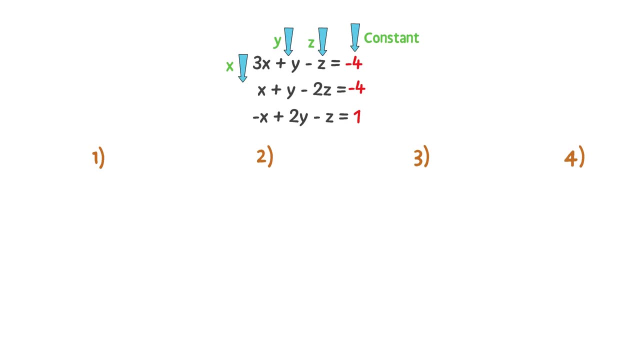 important step and watch it carefully. I take all the coefficient of x column 3, 1 and negative 1.. Then I take all the coefficient of y and z columns as 1, 1 and 2.. Then negative, 1, negative. 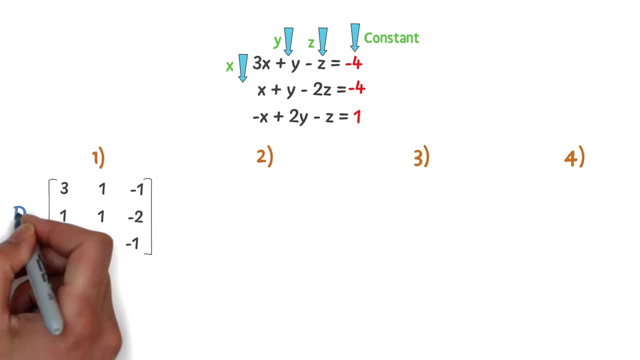 2 and negative 1.. I call this matrix as d matrix or coefficient matrix. Secondly, I will write x matrix or dx matrix. To do so, I will eliminate the coefficient of x column and this matrix and will replace it with the constant column. Let me repeat: I will write: 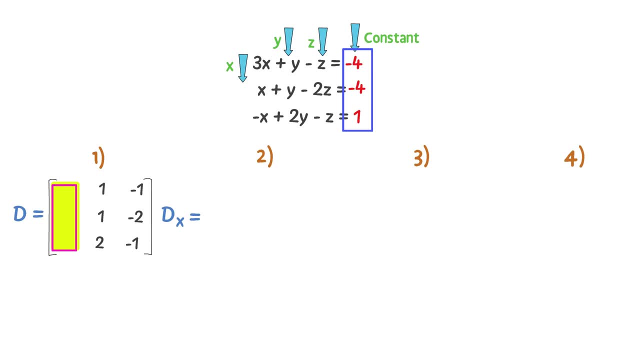 4, 4,. 所以 이렇게繪, I will eliminate the coefficient of x column and this matrix and will replace it with the constant column. So instead of coefficient of x column, I will write negative. 4, negative. 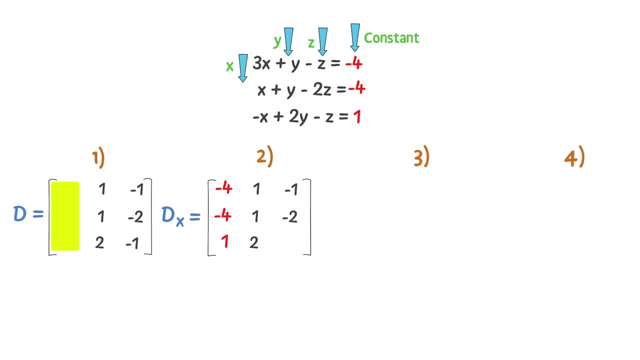 4, 1, then 1, 1, 2, negative 1, negative 2 and negative 1.. Thirdly, I will write y matrix or dy matrix. To do so, I will eliminate the coefficient of y column and will replace 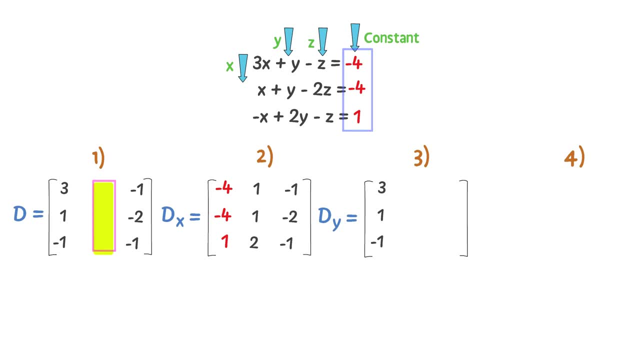 with constant column as 3, 1, negative 1, negative 4, negative 4, 1, negative 1, negative 2 and negative 1.. Fourthly, I will write Z matrix or DZ matrix. To do so, I will eliminate the. 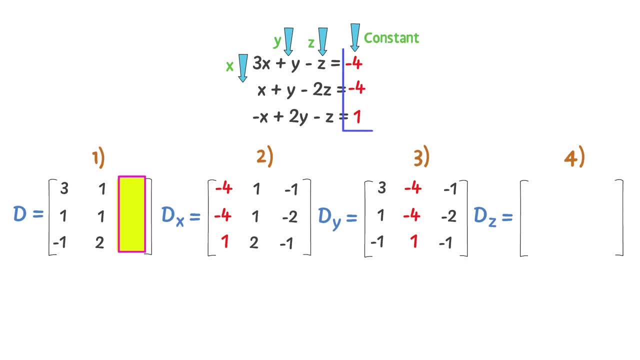 coefficients of Z column and will replace it with the constant column as 3, 1, negative 1, 1, 1, 2, negative, 4, negative 4 and 1.. So I have formed 4 matrices from this system. 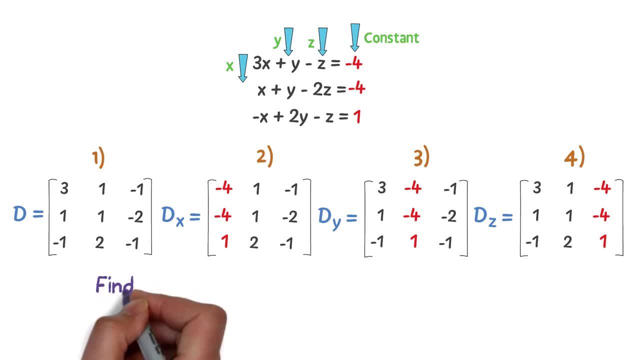 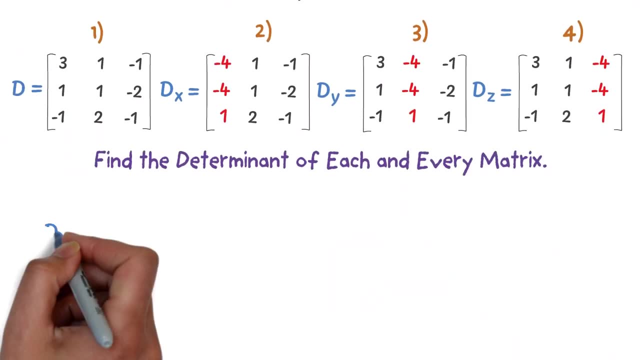 of linear equations. The third and last tip is to find the determinant of each and every matrix. Thus, I will find the determinant of D matrix. Let me take it and write it here. To find the determinant of D matrix, take the first number, which is 3, and write it here. 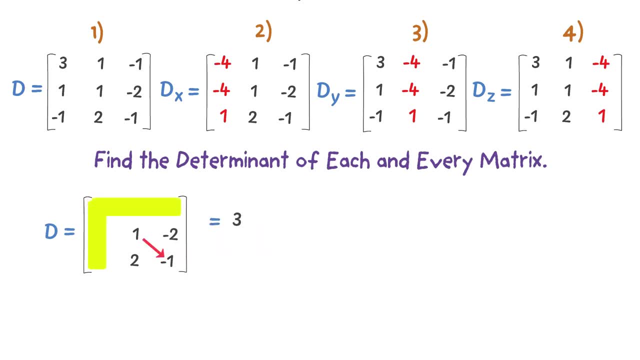 Now hide the row and column of this number. 1 × negative. 1 is equal to negative 1 minus negative 2. X positive 2 is equal to negative 4 minus. take the second number, which is 1, and hide its column and row. 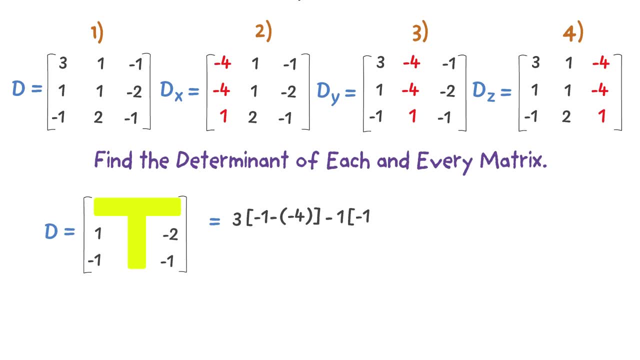 Positive 1 X negative 1 is equal to negative 1 minus negative 2 and to negative 1 is equal to 2 plus. Take the third number, which is negative 1.. and hide its column and row 1 X 2 is. 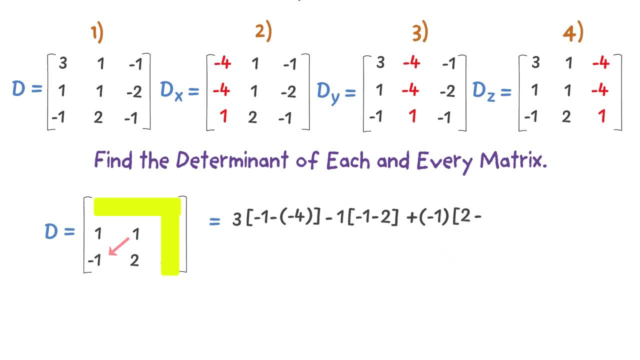 equal to 2 minus positive 1, and to negative 1 is equal to negative 1.. So I write 3 negative, 1 minus, and to minus 4 is equal to positive 4. Negative 1, negative 1 and negative 2 is equal to negative 3. Positive and to negative 1 is. 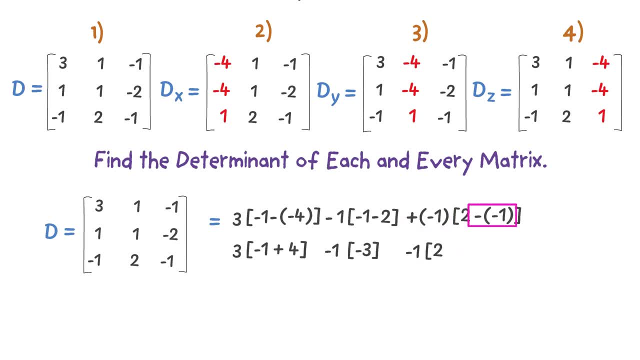 equal to negative 1.. 2 minus and to minus 1 is equal to positive 1.. Thus, negative 1 plus 4 is equal to positive 3. Positive 3 and to positive 3 is equal to 9.. Negative 1 and to negative 3 is equal to positive, 3.. 2 plus 1 is equal to 3.. 3 and 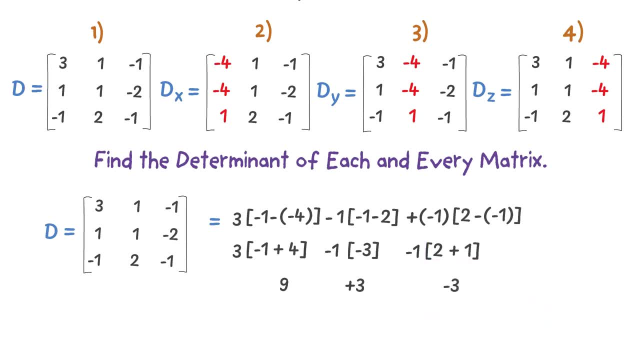 to negative. 1 is equal to negative 3.. Positive 3 and negative 3 cancelled out and we get 9.. So the determinant of D matrix are: D is equal to 9.. Now let me take DX matrix and write it here. 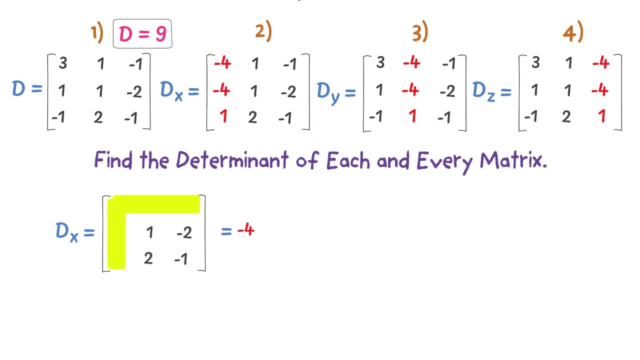 Take negative 4 and hide its column and row. Positive 1 and to negative 1 is equal to negative 1 minus negative 2 and to positive 2 is equal to negative 4 minus. take 1 and hide its column and row. Negative 4 and to negative 1 is equal to. 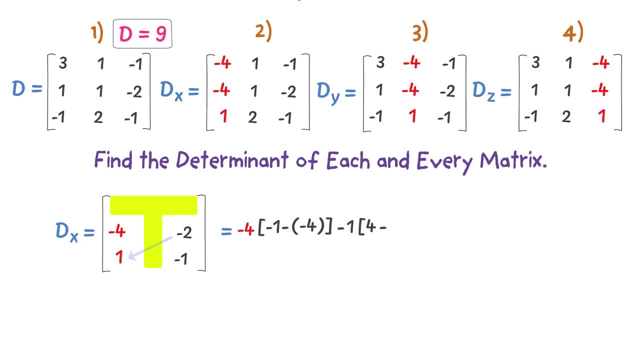 4 minus negative 2 and to positive 1 is equal to negative 2, plus take negative 1 and hide its column and row Negative 4 and to 2 is equal to negative at minus 1 and to 1 is equal to 1.. I get 4. 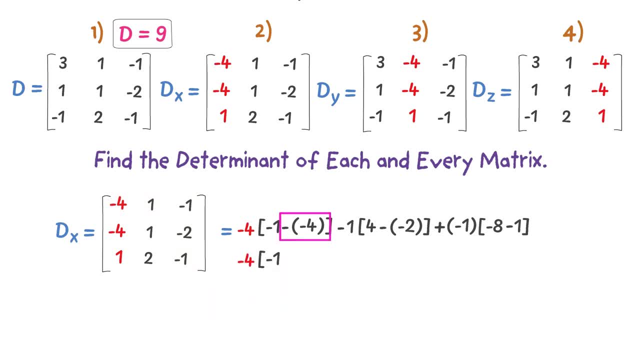 negative: 1 minus and to minus, 4 is equal to positive, 4. Negative: 1, 4 minus and to minus. 2 is equal to positive, 2. Positive and to negative: 1 is equal to negative. 1. Negative at negative, 1 is equal to negative, 9. Negative: 1 positive: 4 is equal to negative, 9. Negative. 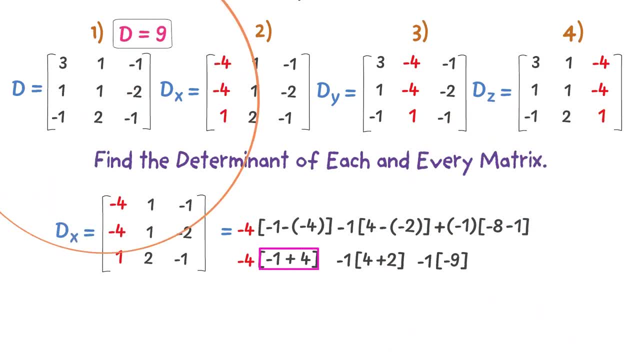 1 positive 4 is equal to negative, 9. Negative 1 positive 4 is equal to negative, 9. Negative 4 is equal to positive, 3. Positive 3 and to negative 4 is equal to negative, 12. 4 plus. 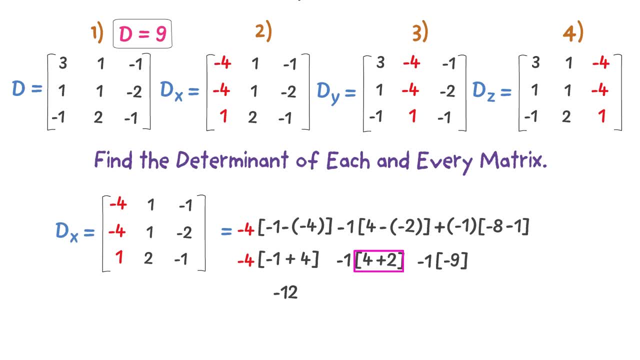 2 is equal to 6.. 6 and to negative 1 is equal to negative 6. Negative 1 and to negative 9 is equal to positive 9.. To calculate negative 12, negative 6 plus 9, I get negative 9.. So 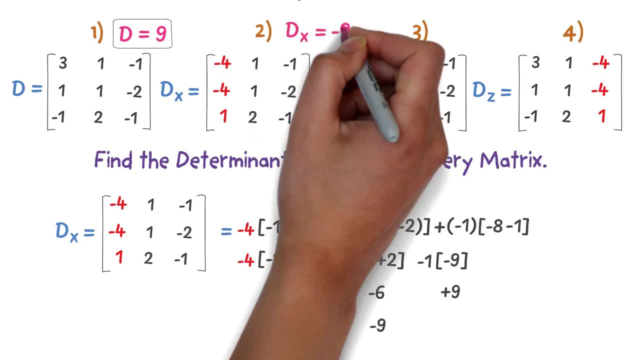 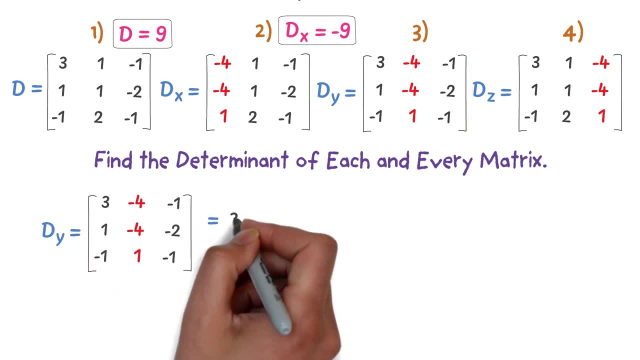 the determinant of X matrix or DX matrix is equal to negative 9.. Negative 9 is equal to negative 9.. Now let me take DY matrix and write it here Again. I take 3 and hide its column and row. Negative 4 and to negative 1 is equal to 4 minus negative 2 and to 1. 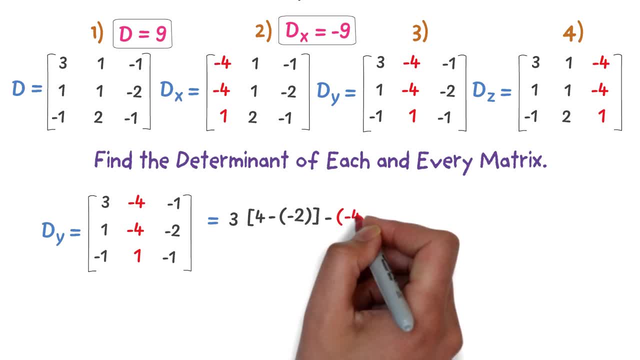 is equal to negative 2 minus. take negative 4 and hide its column and row Positive 1 and to negative 1 is equal to negative 1 minus negative 2 and to negative 1 is equal to positive 2.. Plus, take negative 1 and hide its column and row 1 and to 1 is equal to 1 minus negative. 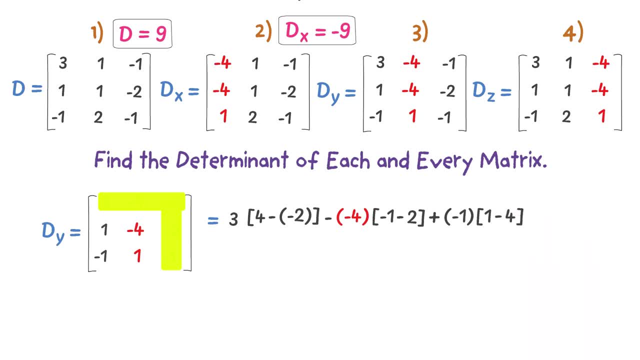 4 and to negative. 1 is equal to positive, 4. I get 3: 4 negative and to negative. 2 is equal to positive, 2. Negative and to negative: 4 is equal to positive. 4. Negative: 1 negative, 2 is equal to negative. 3. Positive and to negative: 1 is equal to negative. 1. Negative: 1- negative. 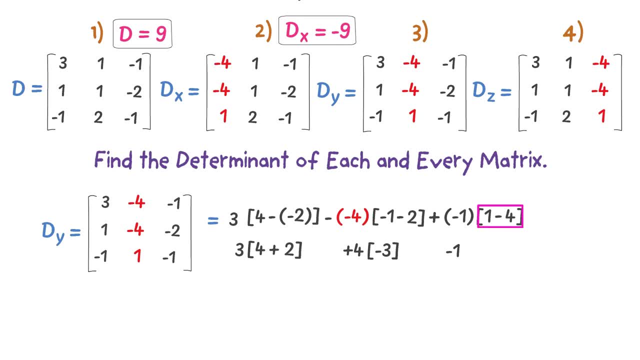 2 is equal to negative, 3. Positive and to negative: 1 is equal to negative, 1. Negative, 1 negative, 2 is equal to negative, 1. 1 minus 4 is equal to negative 3. Now, 4 plus 2 is equal to 6.. 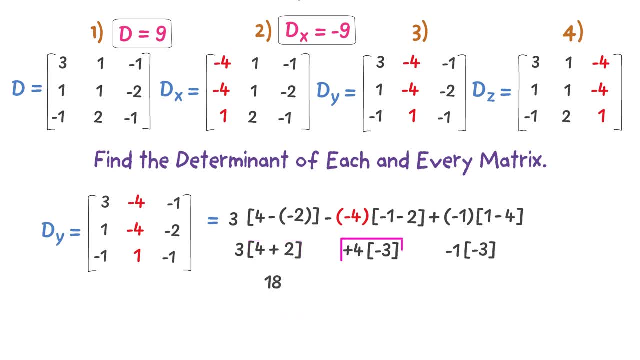 6 and to 3 is equal to 18.. Positive 4 and to negative 3 is equal to negative 12.. Negative 1 and to negative 3 is equal to positive 3.. Here, 18 minus 12 plus 3 is equal to 9.. So 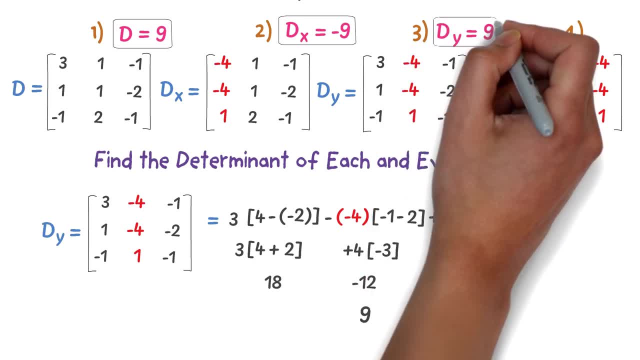 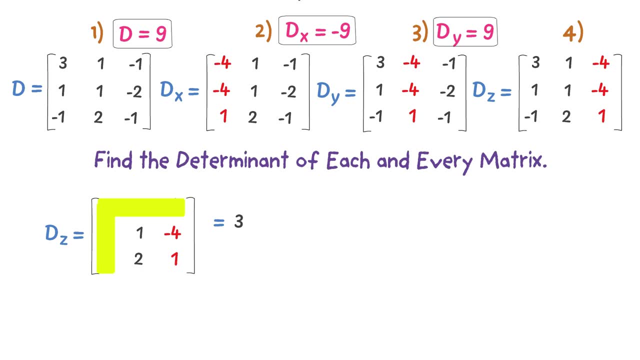 the determinant of Y matrix DY is equal to 9.. Lastly, let me take the Z matrix. I take 3 and hide its column and row 1 and to 1 is equal to 1 minus negative 4 and to positive 2 is equal to negative 8 minus. take 1 and hide its column and row 1 and to 1. 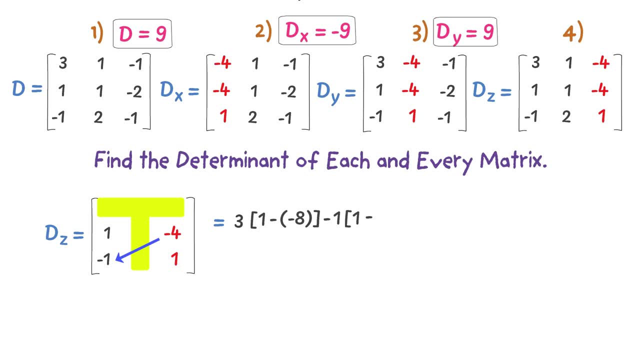 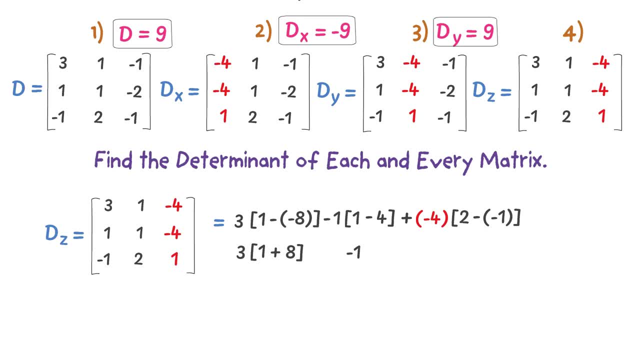